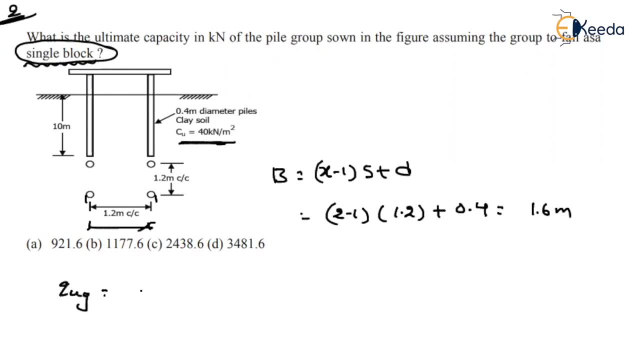 So what about the capacity in group? That will be equal to end bearing resistance. What is the end bearing resistance? That is nothing but a cnc into ab plus. what about the frictional resistance? That will be equal to alpha into surface area as into frictional resistance. 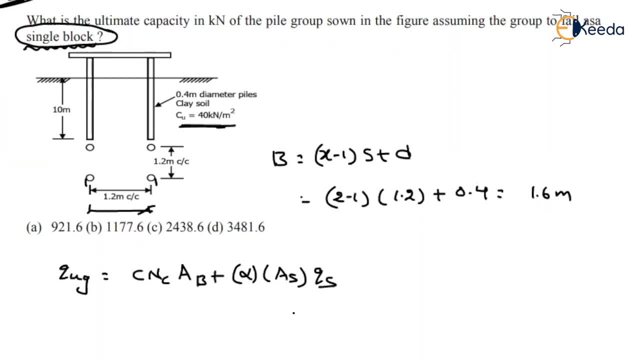 Let us say q-test. Now what about the c value given Coag, and whatever it may be, it is 40. So that will be equal to 40.. Did they have given nc value? No, That means resume it as 9.. 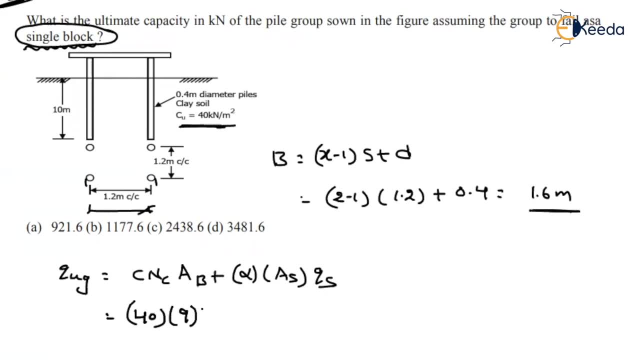 What about area if it is failing by group? 1.6 meter, So if it is like a square shape. so what is the square area? 1.6 square plus? what about the adhesion factor? 0.4 into whatever the shear resistance? again it is 40. 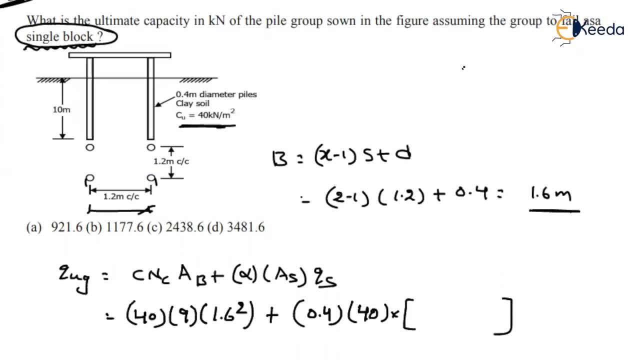 into what about the surface area? So if it is in the form of square, what about the circumference length Each sets? we are having 1.6 meter, as it is a square. That is why I will say 4 into 1.6, into what about the length of the pile? 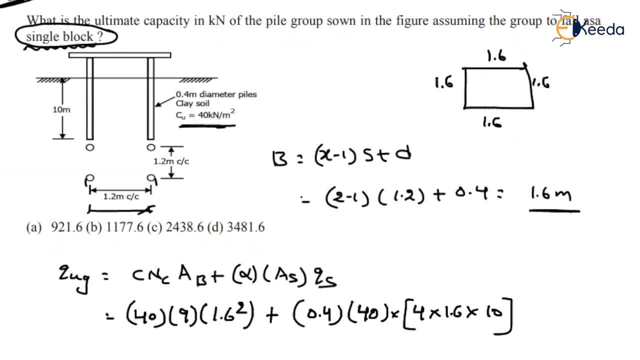 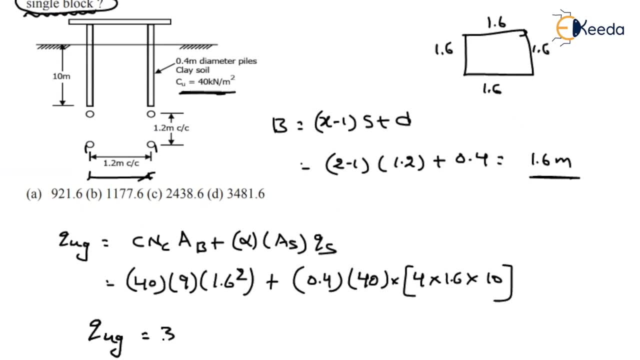 10 meter. If you solve this, you will get the capacity of a pile group. That will be is equal to 3481.6 kilonewtons. Answer is there. Yeah, That is the correct answer, Suppose if it is a numerical, you have to enter. 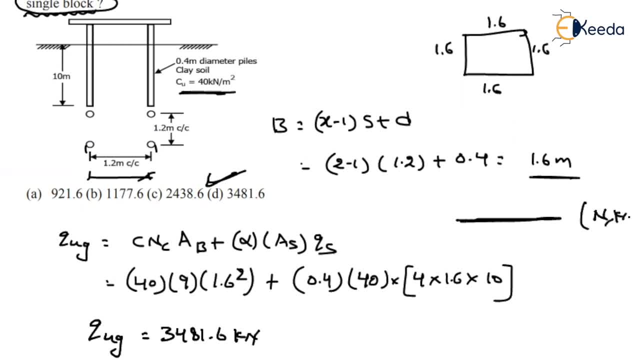 You have to see whether they are asking capacity in Newton, kilonewton, or whether they are asking in meganewton, Corresponding to the unit. you have to enter the answer. If it is directly, if you have to pick the answer directly, we can idealize in our mind. 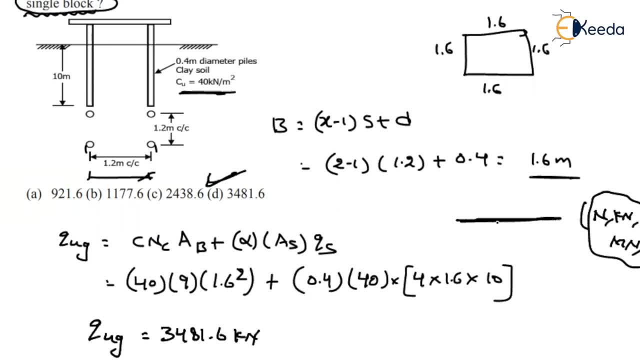 Okay, Whether they are in kilonewton, meganewton, But if they are asking a numerical answer type, we have to see the unit Understood. Suppose, if I want to express this in meganewton, what is the answer? 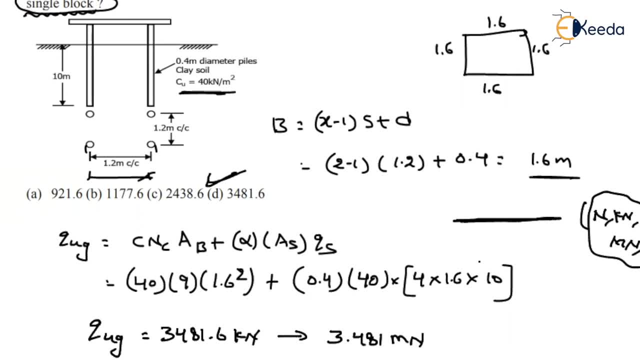 3.481 meganewton. So is there a difference, right? If we enter 3481.6,, if we enter 3.481,? there is so much of difference. So if you are entering numerical type questions, please make sure in which unit you are representing. the answer. Okay, Thank you.